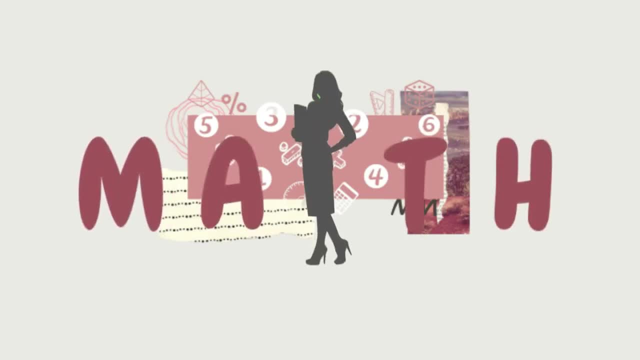 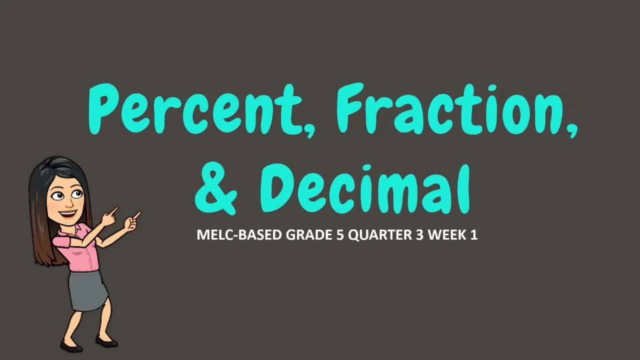 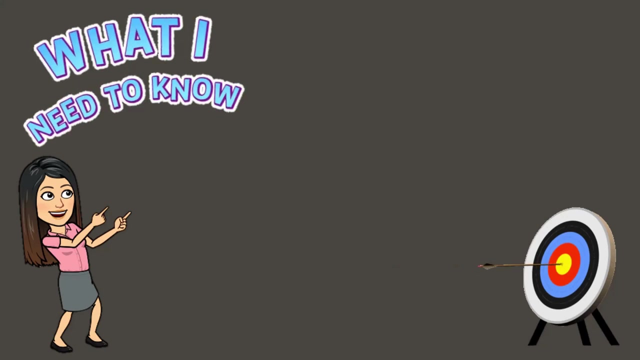 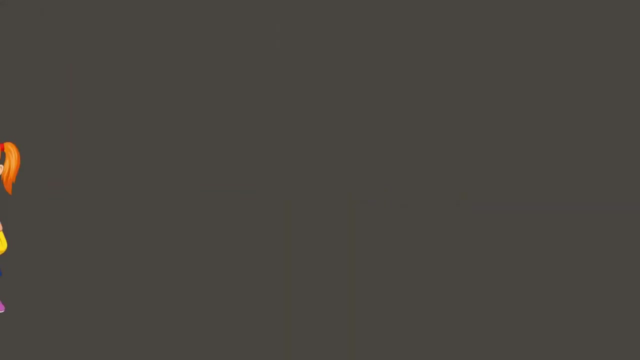 Percent, Fraction and Decimal. Good day students. Welcome back to my classroom For today's lesson. you are going to learn how to visualize percent and its relationship to fractions, ratios and decimal numbers using models. Let's begin. Let's meet Marie. 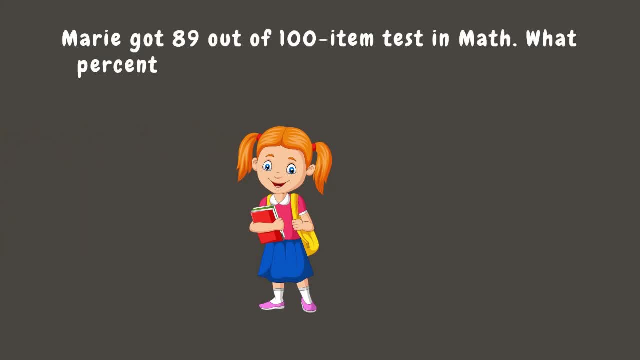 Marie is a grade 5 student. She got 89 out of 100 item tests in math. Now what percent of the tests did she answer correctly? Here we are asked to get the percent of the tests. Marie answered correctly, But wait, do you know what percent means? 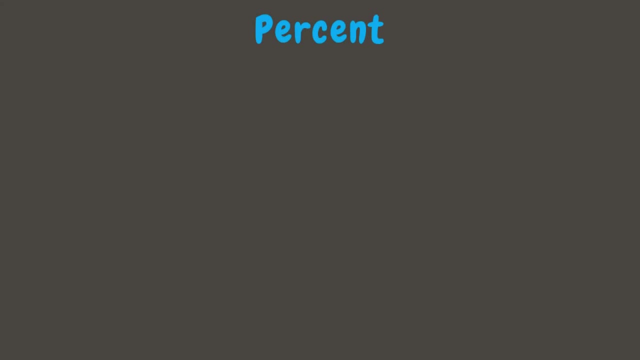 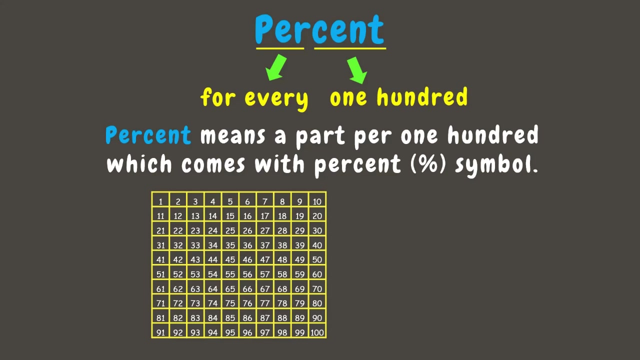 In the word percent per means for everything, While cent means 100. Therefore, percent means a part per 100, which comes with percent symbol. For example, a figure here is divided into 100 parts. If 100 parts are shaded, the shaded part represents 100%. 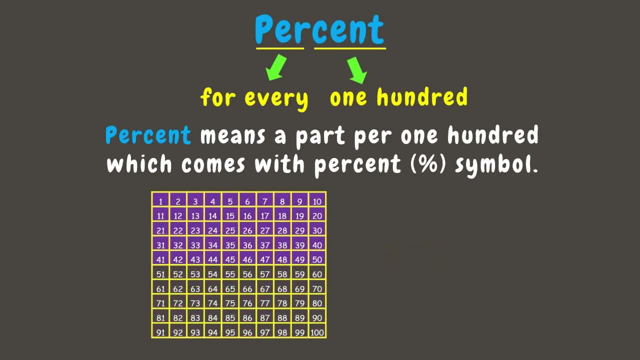 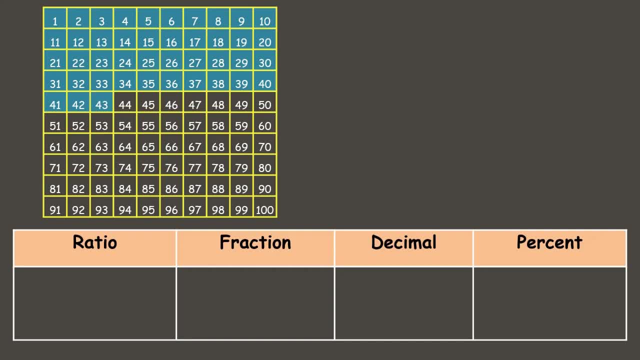 So, iniseen ratio, we can compare the number of shaded parts, which is 43, to the total number of parts, which is 100,, which gives us the ratio 43,S to 100.. In fraction, we can simply write this as 43 as the numerator and 100 as the denominator. 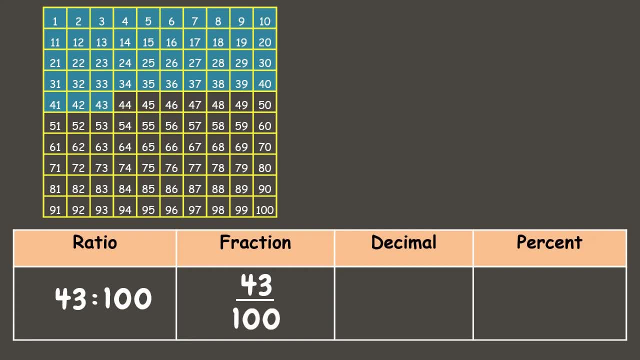 In decimal, since the fraction is 4,300, we can write this as 0.43,, while in percent it would be 43%. Well, in decimal, since the fraction is 4,300, we can write this as 0.43,, while in percentage it would be 43%. 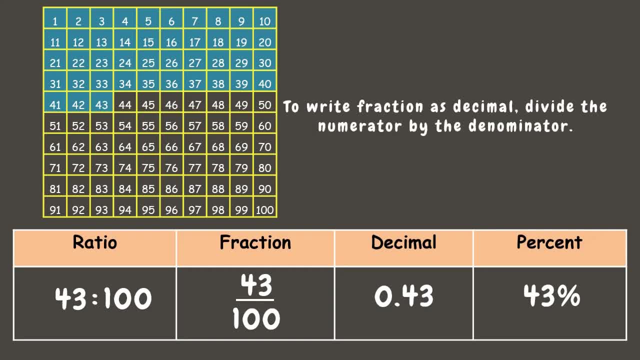 Now to write a fraction as decimal, we can simply divide the numerator by the denominator. Let us try. We have here our fraction 43 out of 100 or 4300.. Now let's divide 43 by 100.. Since 43 is smaller than 100, let us add 0.0.. 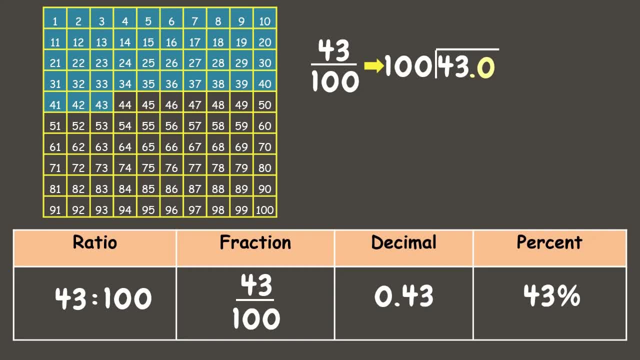 We have 430 divided by 100. That is 4.. 4 times 100 is 400.. And if we subtract this, we'll get 30.. Since 30 is smaller again than 100, let us add another 0.. 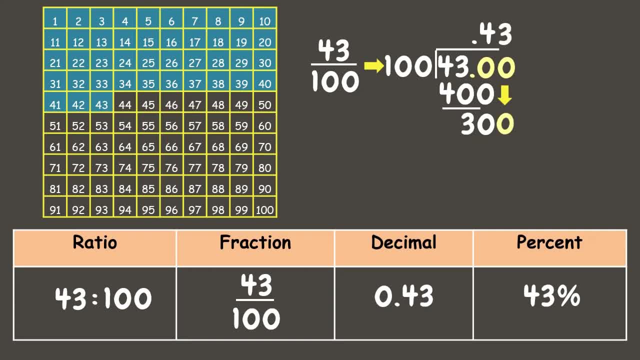 Now, 300 divided by 100 is 3.. 3 times 100 is 300.. And if we subtract this, it's 0.. Don't forget to put the decimal point aligned from the decimal point in our dividend. Now our final answer is 0.43. 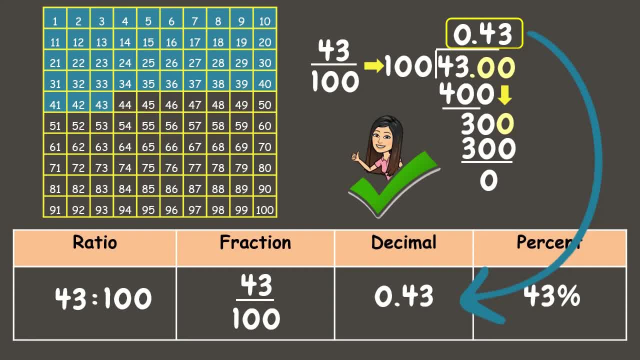 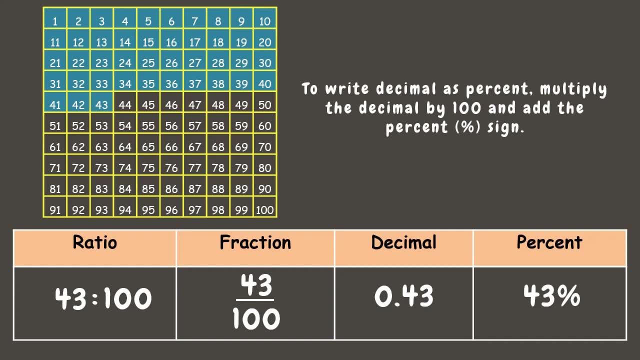 Which is the same as our answer. Also, to write decimal as percent, we can simply multiply the decimal by 100 and add the percent sign. Let's try. We have here decimal 0.43 or 4300 times 100.. 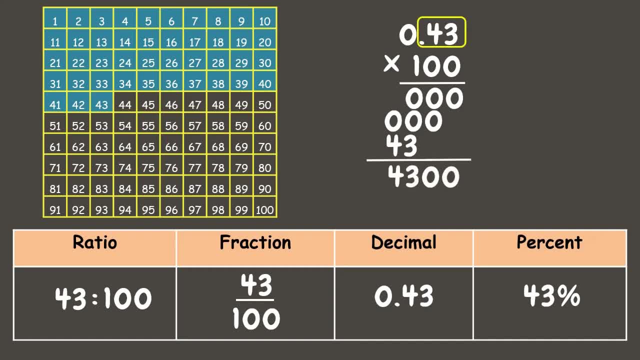 Since we have two decimal places here, let's put the decimal point two places to the left. There you go. Now we have 43 and add the percent sign, That will be 43 percent. Same as our answer earlier. There is also a shorter way to write decimal as percent. 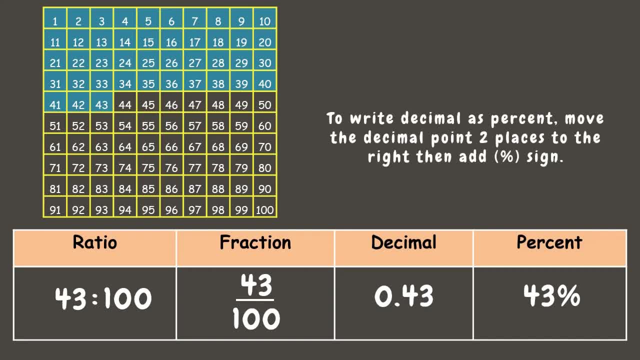 It is to move the decimal point two places to the right, then add percent sign. So if we have 0.43 or 4300, simply move the decimal point two places to the right, then add percent sign. That will also be 43 percent. 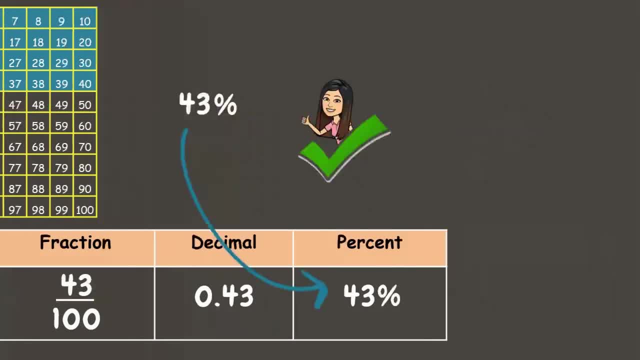 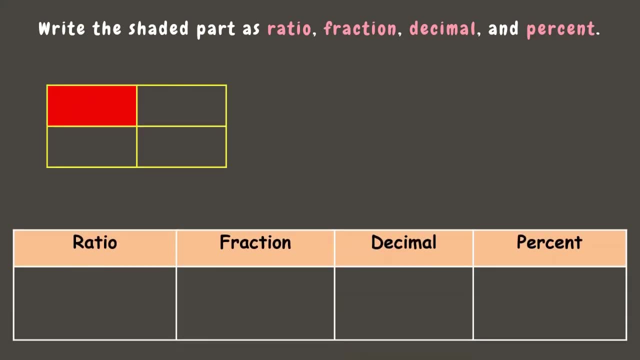 Wonderful. Now let's have more examples. Write the shaded part as ratio, fraction, decimal and percent. Let's get its ratio first. Here we can see that there is one part shaded, which will be our first quantity, out of four parts, which will be our second quantity. 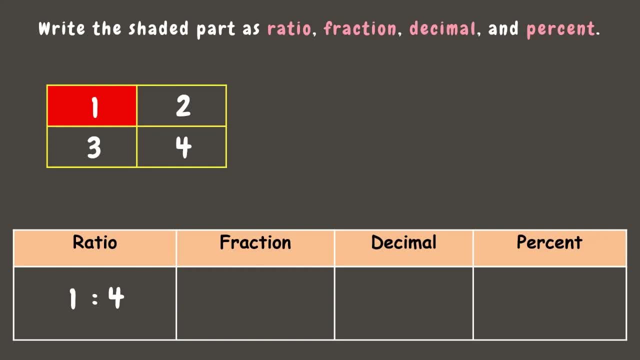 Therefore our ratio would be: 1 is to 4. And fraction, it is 1.. 1. fourth, For decimal, we need to divide the numerator by the denominator, So that will be 1 divided by 4.. Since 1 is smaller than 4, let us add 0.0.. 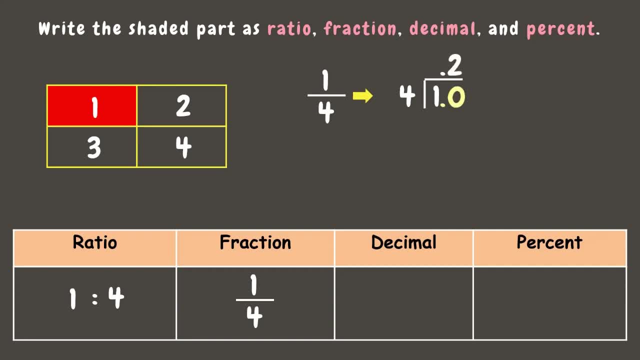 10 divided by 4 is 2.. 2 times 4 is 8.. If we subtract this, this will be 2.. Since 2 again is smaller than 4, let us add another 0. We have 20 divided by 4.. 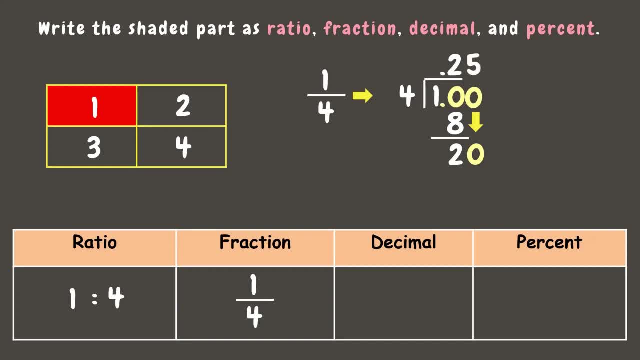 That is 5.. 5 times 4 is 20.. And if we subtract this it will be 0.. Again, don't forget to write the decimal point aligned from our dividend. Now our answer is 0.25 or 2,500. 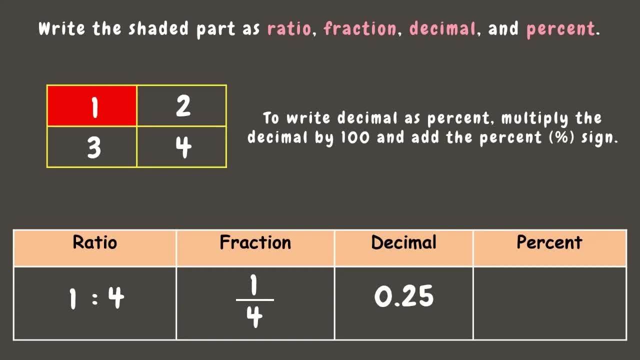 Now let's convert this decimal into percent by multiplying this by 100.. 2,500 times 100.. Since we have two decimal places here, let's put the decimal point two places to the left. There you go, And then add percent sign. 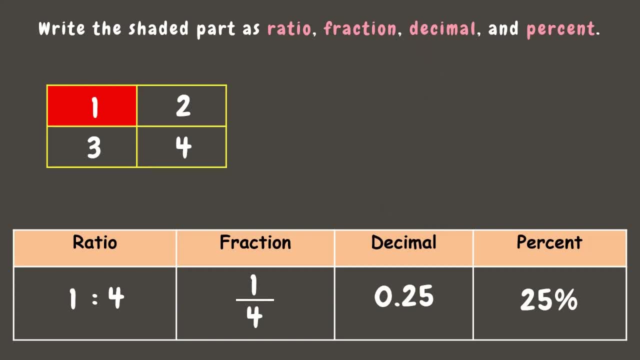 We'll have 25%. Or we can use the shorter way, which is to move the decimal point two places to the right. Let's try. We have 0.25.. Move the decimal point two places to the right And we'll get 25%. 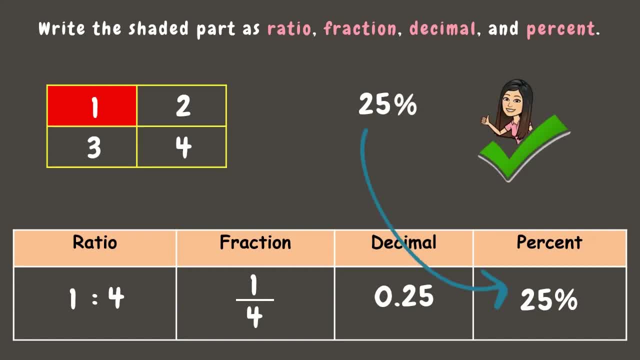 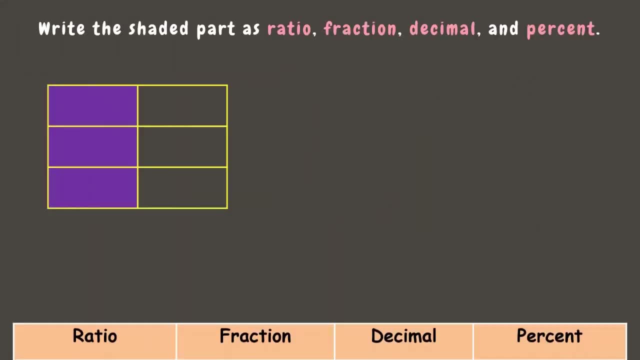 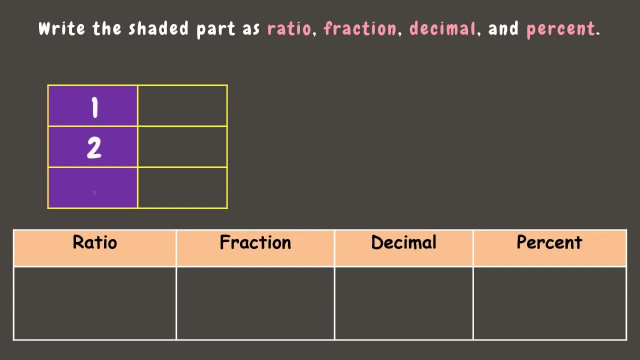 Which is the same as our answer. Great job. Now let's have one last example. Again, let's write the shaded part as the ratio: fraction, decimal and percent. Let's get its ratio first. Here we can see that there are three parts shaded, which will be our first quantity, out of six parts, which will be our second quantity. 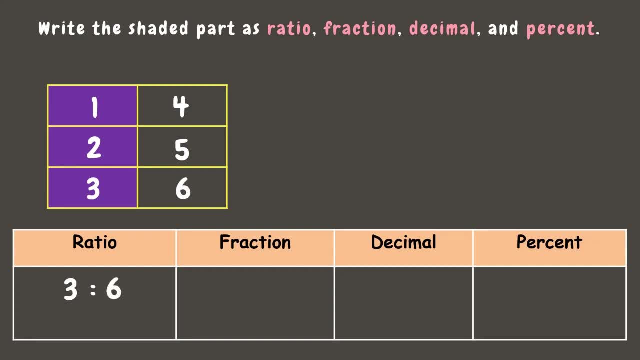 Hence the ratio is 3 is to 6. And fraction it is 3 is to 6. And, as you can see, this fraction can still be reduced to its lowest term by dividing it by its GCF 3..